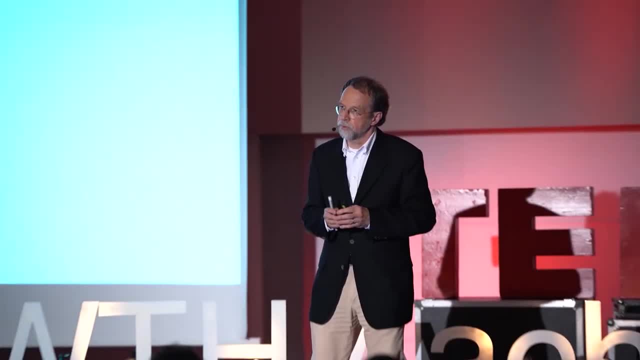 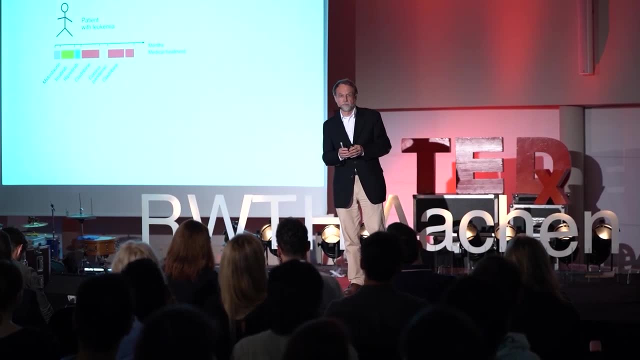 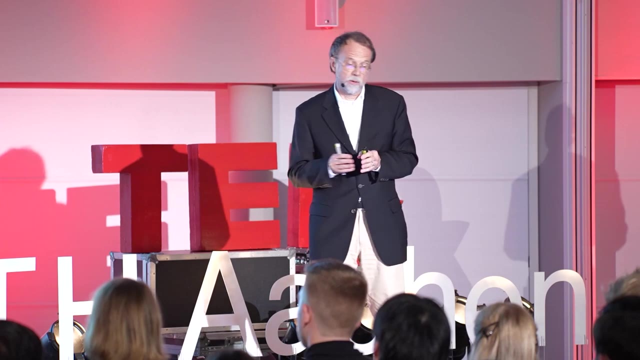 mitostaurine, which is the standard therapy for this particular disease, but this didn't work, So he was then treated with imatinib, which also didn't work. He was then treated with ripritinib, which also didn't work, And then the clinicians put him on cytostatic therapy. 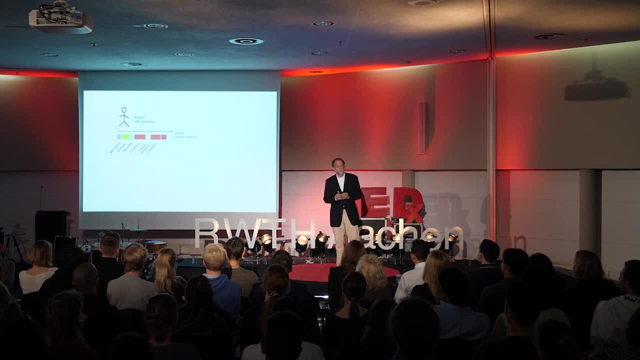 and they worked a little bit. so there was impassionment And the patient then hesitated to show up in the clinics because of the pandemic situation. When he came back, his health status was really bad and he was again put on cytostatic therapy. 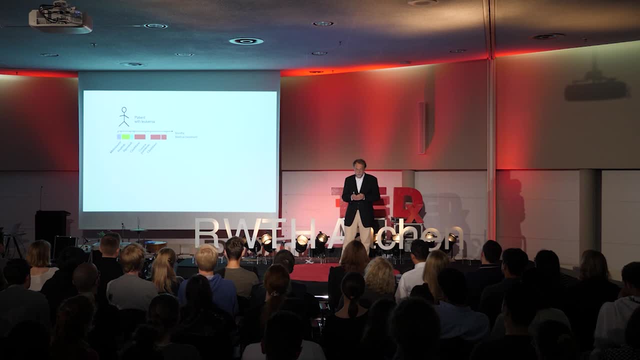 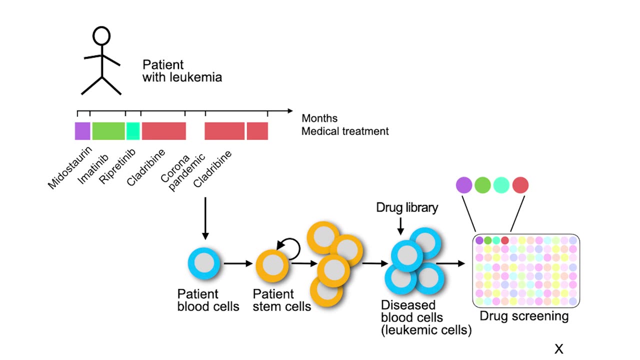 This was without any effect, And this was about the time when we decided to make stem cells. So we took patient blood cells and converted them into patient stem cells and then grow these patient stem cells to high cell numbers and differentiated them into the disease blood cells, the leukemic cells, which were then subjected to drug screening. 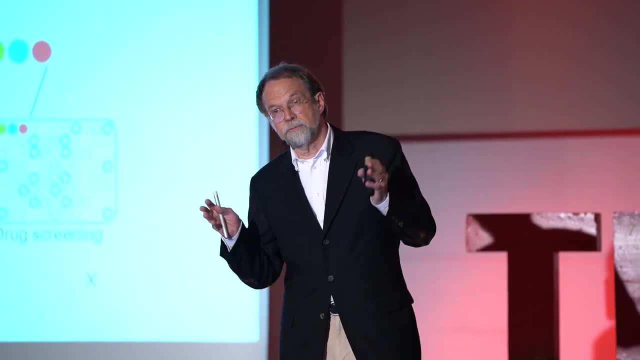 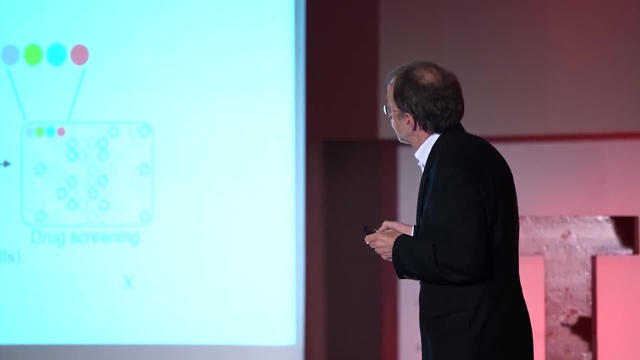 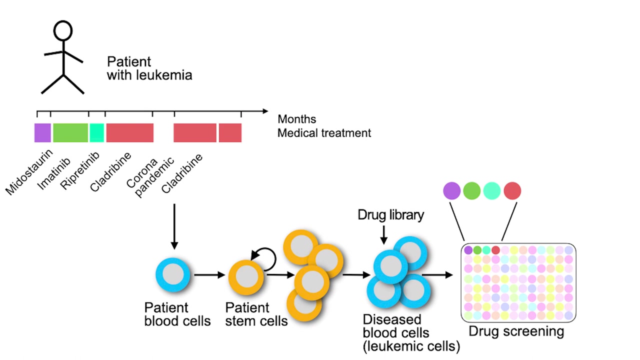 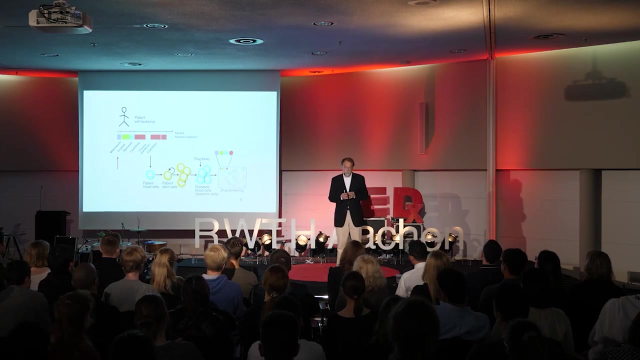 with the intention to identify a drug which would now specifically kill the leukemic cells. So the concept is that, instead of using drug after drug in this more consecutive treatment, we test many drugs simultaneously and parallel in a very short period of time to come up with a drug. 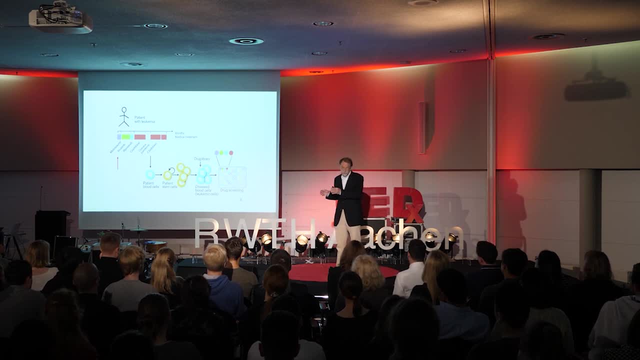 which would work on the disease cells in the screen and should therefore also work on the disease cells in the patient. But unfortunately we were late and the patient died So before we were able to finish the screen. So actually we should have started much earlier. 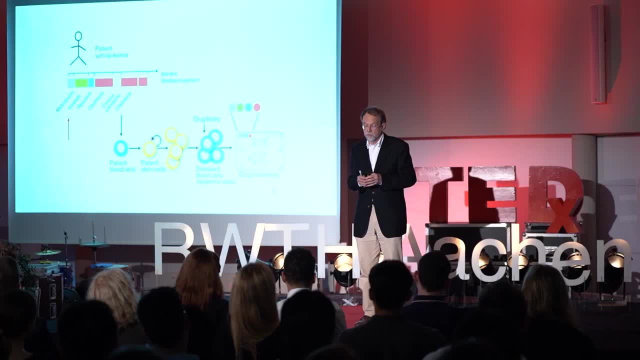 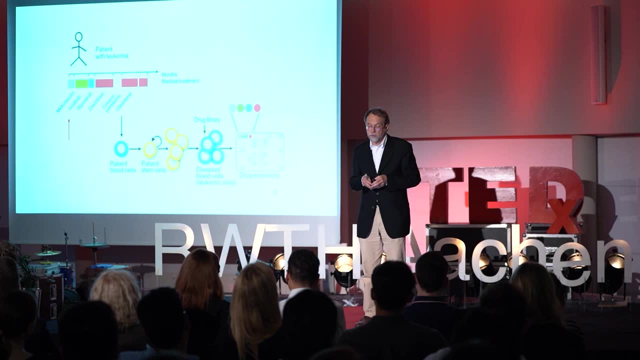 At the beginning, when the patient showed up in the hospital, to start this screening and to come up with the right and tailored drug therapy from the very beginning, Because you might think about this, This is a patient, but it might be yourself, It could be a member of your family, your brother. 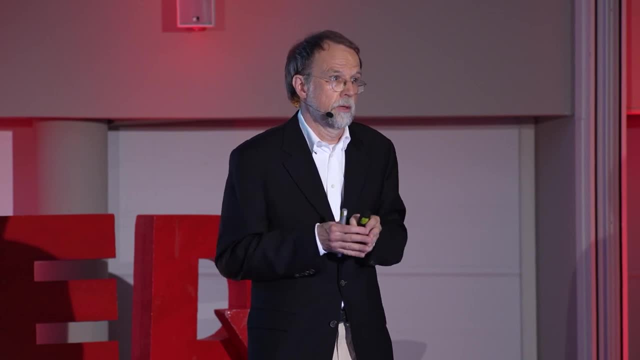 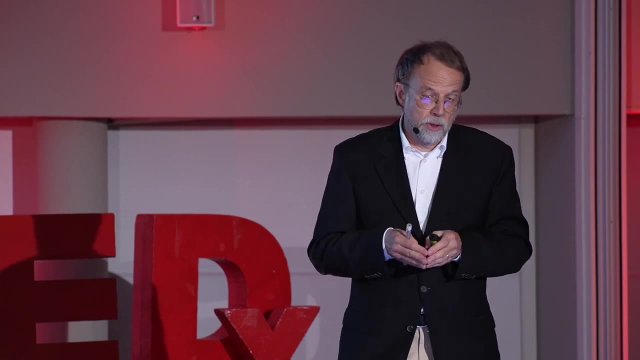 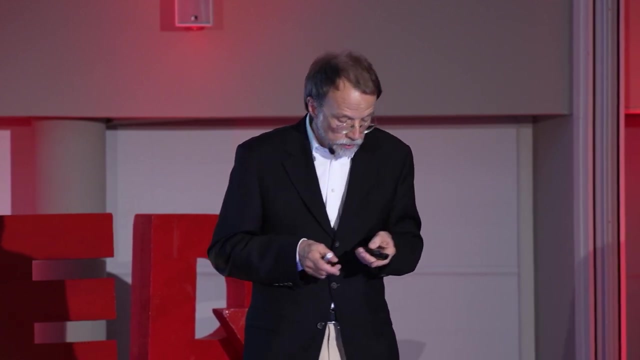 your sister, your mother, father or a friend or colleague? And the key question is: why do drugs work on some patients and fail in other patients, although these patients have essentially the very same disease? And the answer is pretty simple: because people are different, Patients are different. 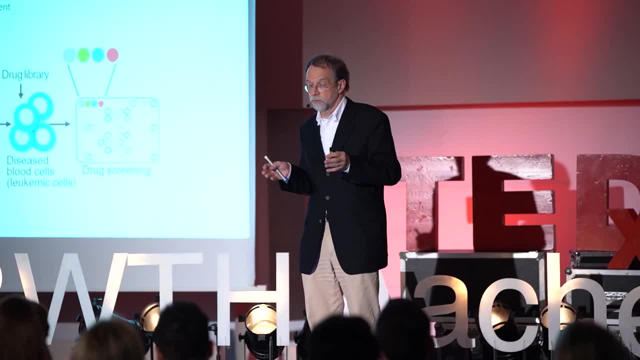 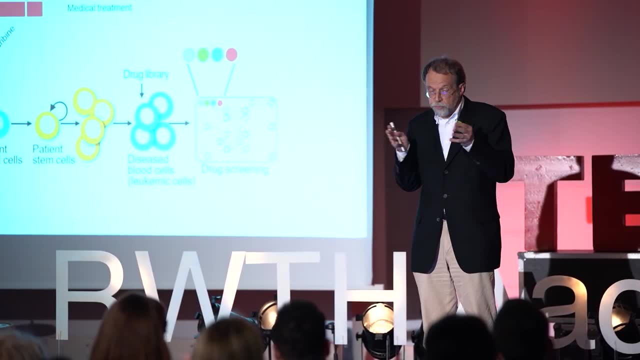 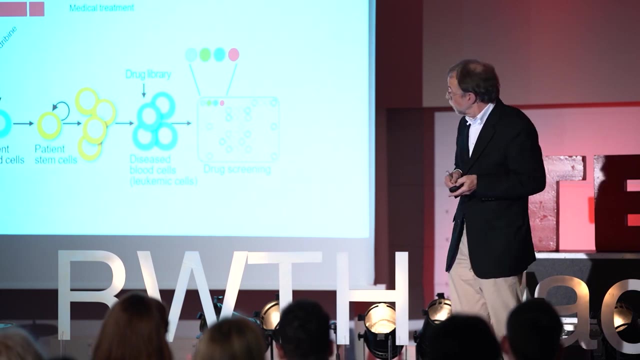 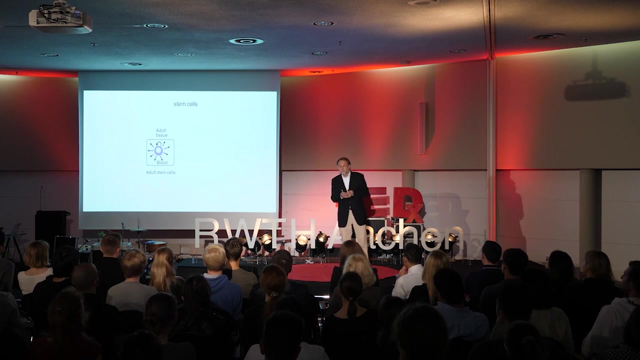 And this means that even the same disease can be different in different patients, And this calls for both disease and patient tailored therapy, which we call precision medicine or personalized medicine, And here stem cells and CRISPR come in. So what are stem cells? So I'm a stem cell biologist and we are very fascinated about stem cells. 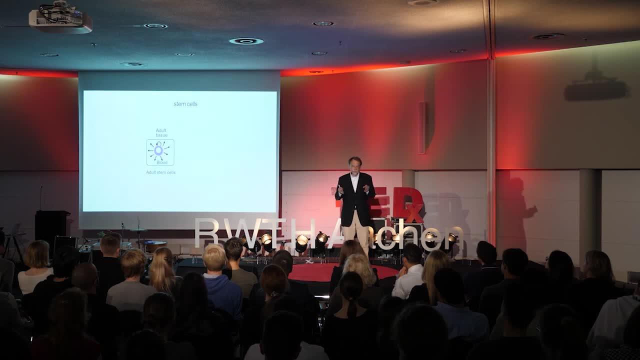 because they have these unique properties and cool cells to work with. But they're actually very interesting cells because they combine two properties in one cell. One property is to grow. So a stem cell will divide, generate two stem cells, four stem cells, eight stem cells, 60, millions of stem cells. 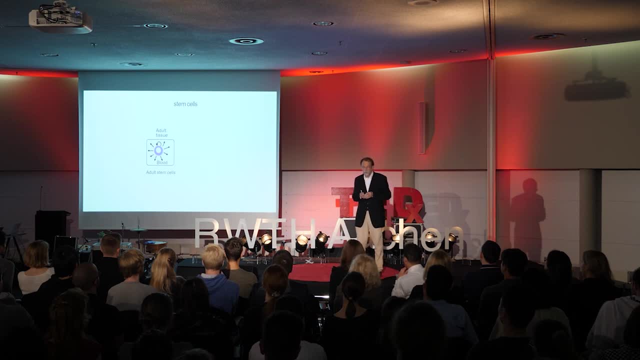 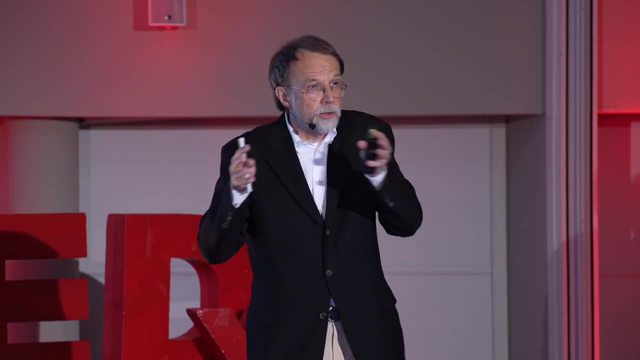 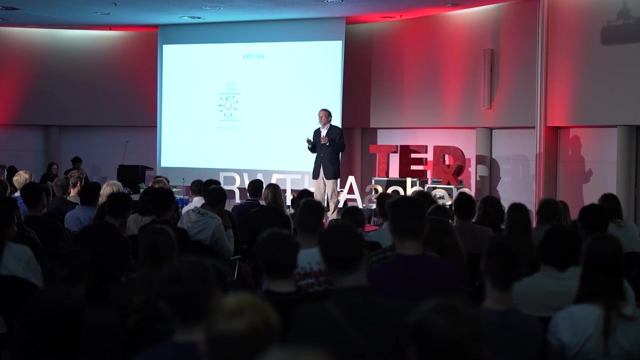 And while keeping still the stem cell identity. But the stem cell can also leave this state of stem cell identity and differentiate and acquire another identity. For example, a blood stem cell can differentiate into all cells we have in blood, so the white and the red blood cells. 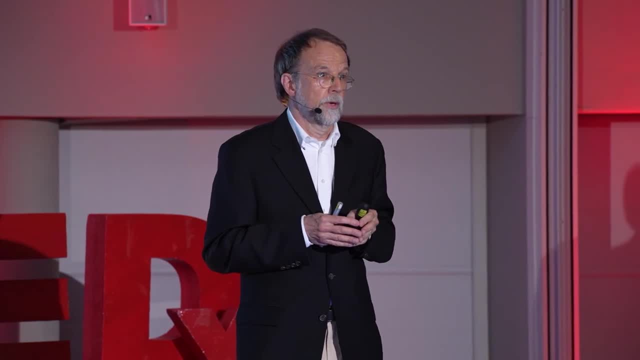 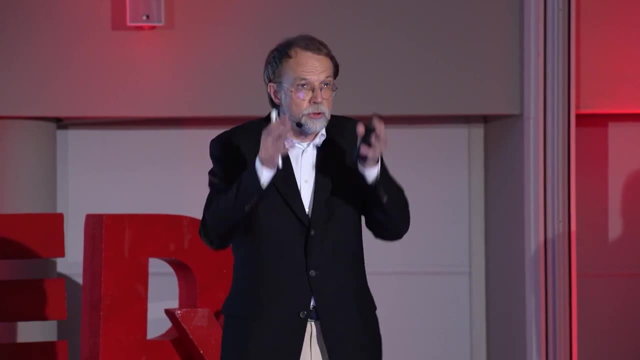 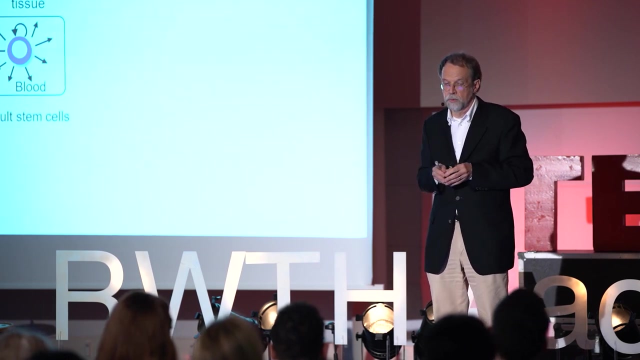 Or liver stem cell can differentiate into liver cells And this property is confined the particular organ or tissue. So a blood stem cell will always give blood and not liver, and a liver stem cell will always give liver and not blood, But we have in the embryo another. 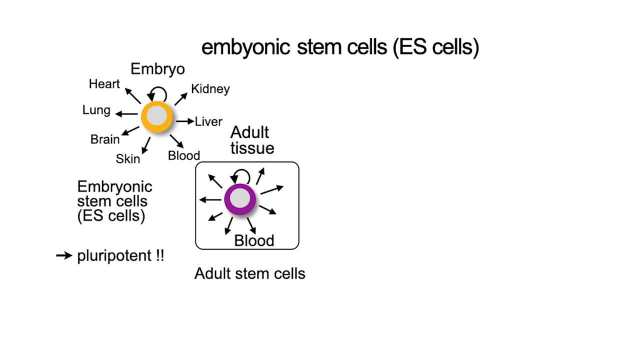 cell type, which is an embryonic stem cell, or an ES cell, which is even more potent. We call it pruripotent because, when the embryo develops, these cells develop into cells of various tissues of the kidney, the liver, the bladder and so on. This is what we refer. 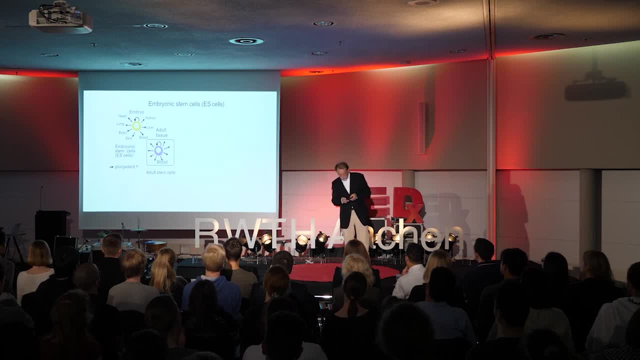 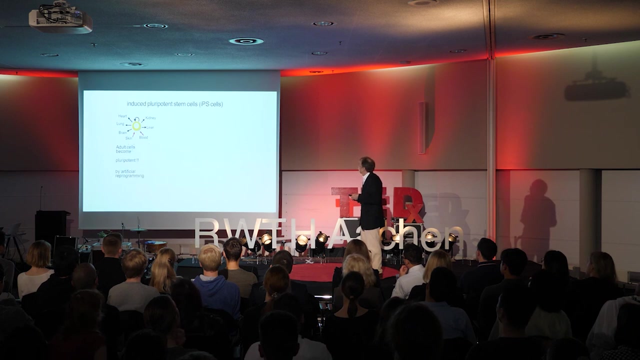 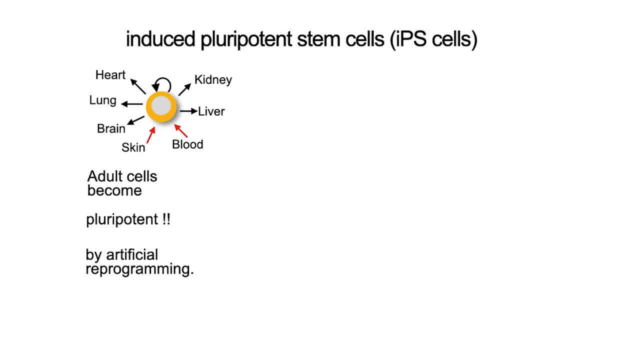 to as pruripotency. And what is even more surprising is that this process, that a pruripotent cell can develop into various tissue cells, this process can be reversed And an adult cell can artificially reprogram to become pruripotent. We refer to this as 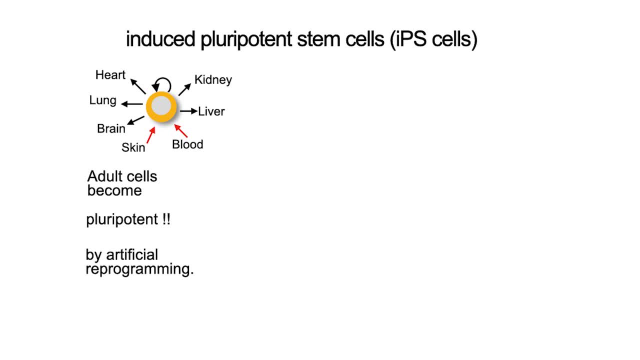 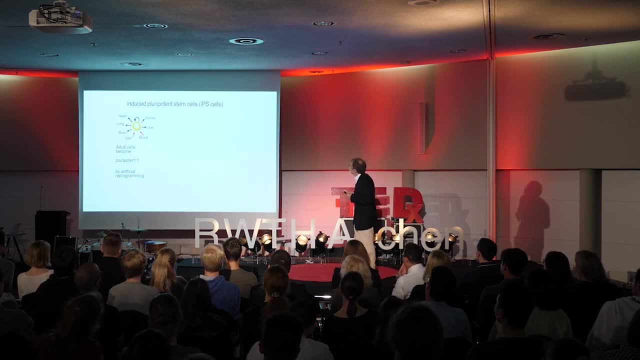 as an induced pluripotent stem cell or an iPS cell. And when I'm going to talk about stem cells in the following, I'm referring to this induced pluripotent stem cells or iPS cells, And we can use now this trick. 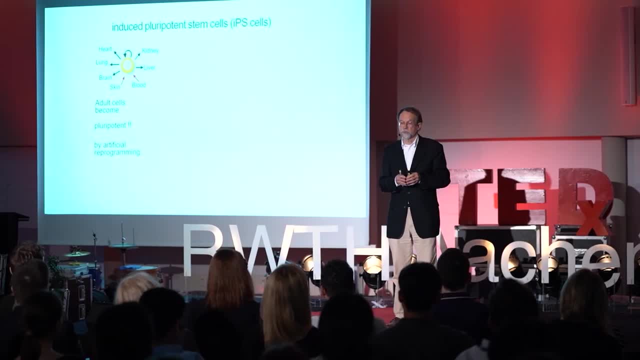 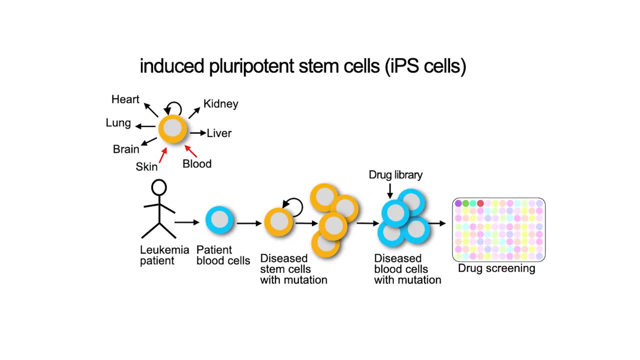 to make patient and disease-specific stem cells for dark screening. So what we do is we take patient cells and subject them to this procedure, this reprogramming procedure, to generate stem cells with the mutation, because these stem cells pick up the disease-specific or disease-associated mutations. 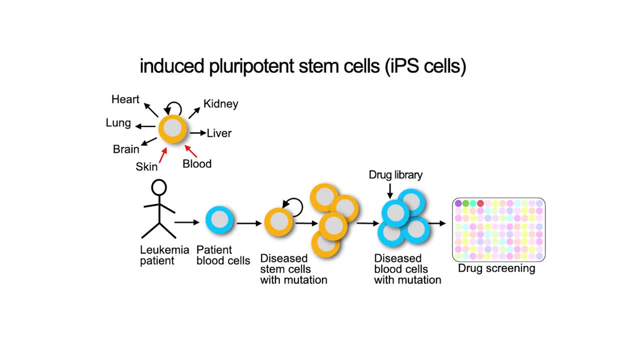 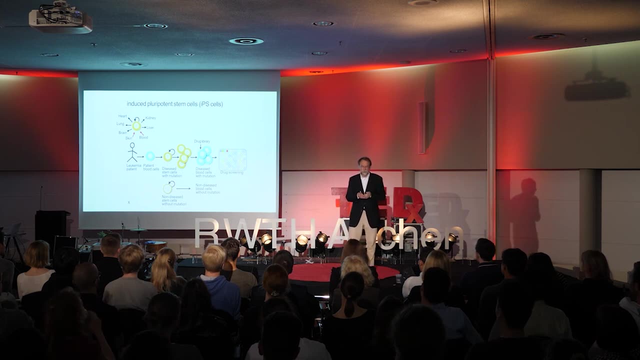 but also the patient-specific genetic program, And we can grow these cells into a larger number and convert them in the diseased blood cells and use them for dark screening, as I showed you before. Well, we need a control which is a non-disease. or at least a healthy cell without mutation, because we want to have a drug which works on the mutated diseased cells but not on the non-mutated healthy cells. And in leukemia the mutations, like in many cancers, are acquired mutations. 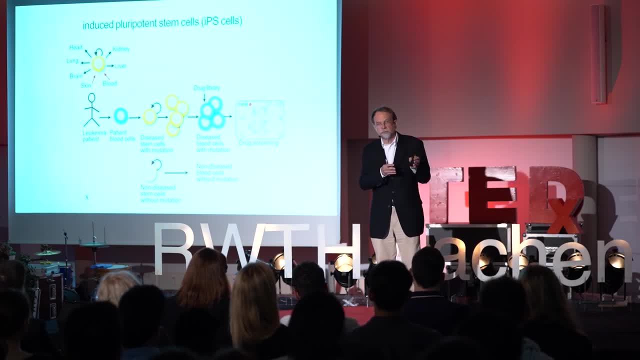 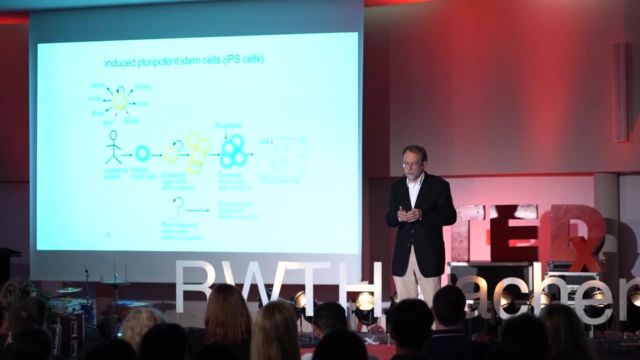 So they occur only in the diseased cells and not in the non-diseased cells. So in a patient, a leukemia patient- has also non-diseased cells and we can also use these non-diseased cells, these healthy cells. 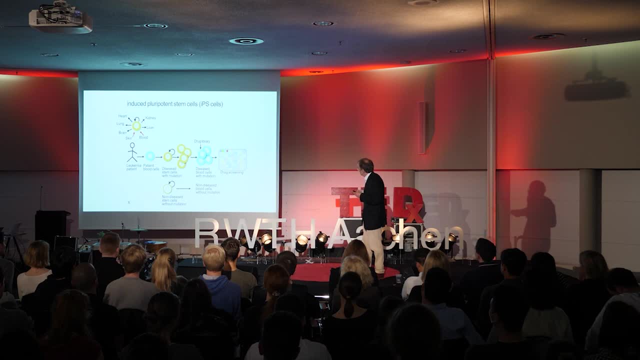 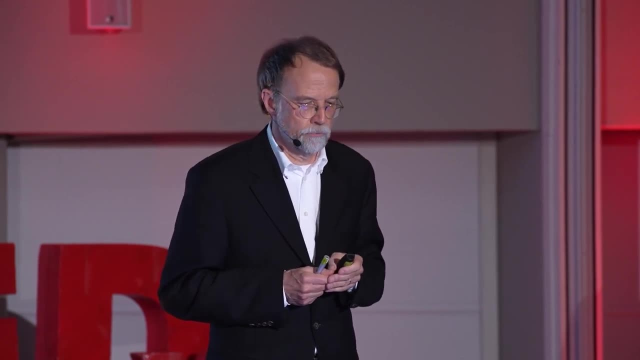 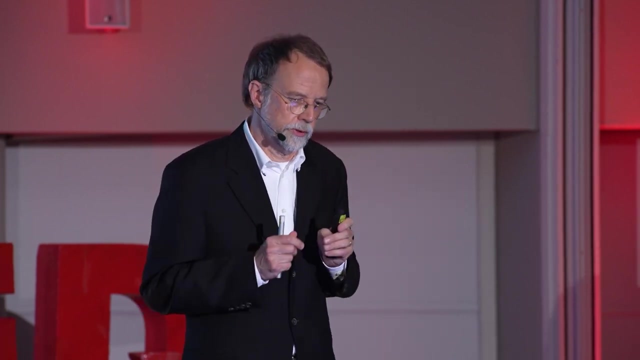 to reprogram them into stem cells and generate the non-diseased blood cells for our control in our drug screening. So the take-home message at this point is that we use this trick to convert a patient cell into a diseased and a non-diseased patient cell. 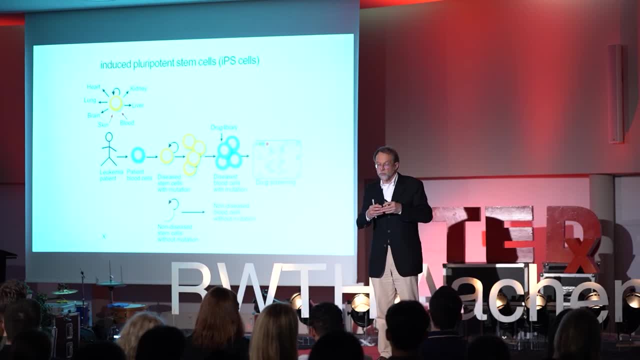 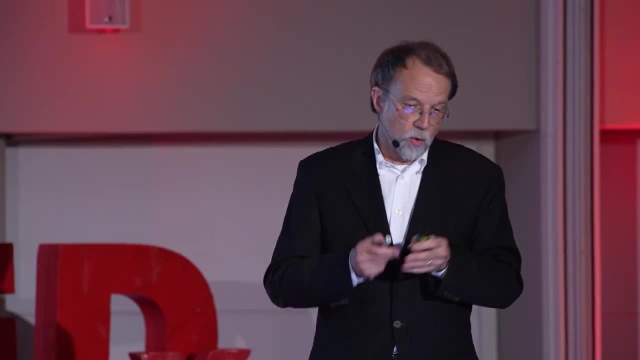 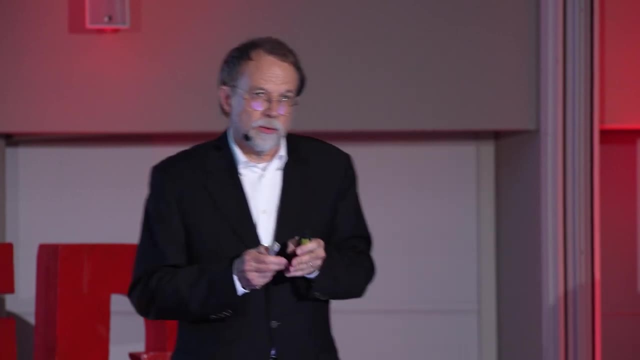 with and without mutation, to screen for drugs, to identify drugs which we would expect to work in the diseased cells of the screen and then also should work in the diseased cells of the patient. This gets me to my second example, which is on pain. So we all experience pain. In most cases it's an unpleasant experience, But there are even people who don't have pain. so they have mutations in ion channels and no pain. So are these lucky people? No pain, no problems. It's not that simple. because you might hurt yourself without noticing. So it's pretty dangerous to have no pain. So pain is a rather useful sensor. But what happens if this pain sensor runs wild and generates a signal of constant pain or generates the signal of hyper-intensive pain? 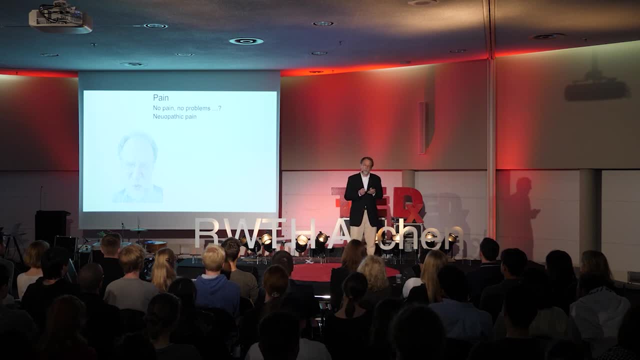 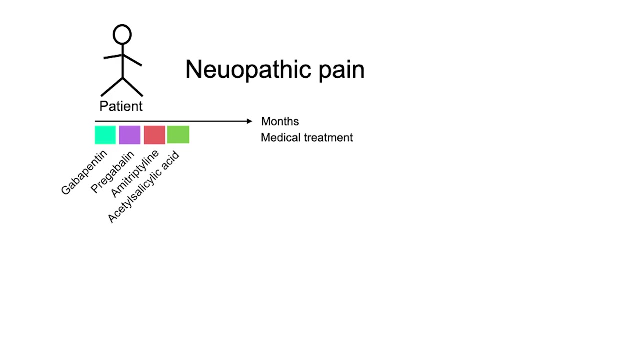 So there are patients who would sense what we think is warm and comfortable as hot and unbearable, And this is what we call the neuropathic pain. And neuropathic pain occurs in patients. Here I show you one patient And she got treated with different compounds, drugs. 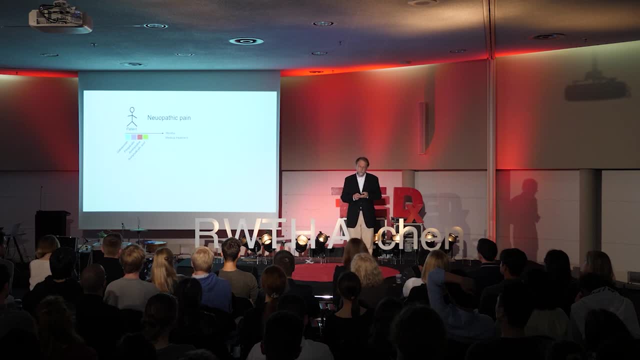 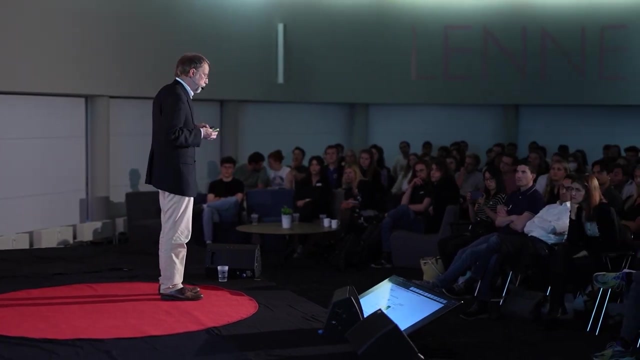 which were all non-effective or have been discontinuous because of severe side effects, And therefore this patient was then subjected to stem cell drug screening. So a patient blood cell was taken and then converted into the diseased stem cell. These diseased stem cells were amplified. 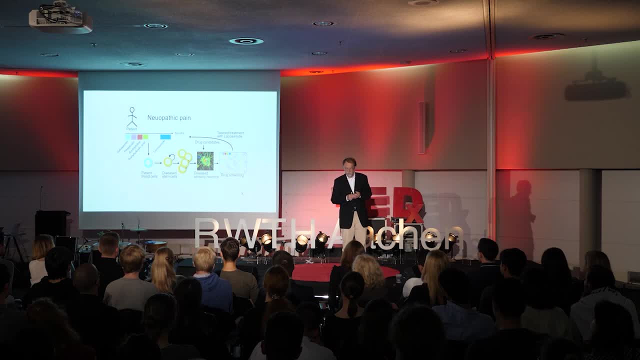 converted into sensory neurons. These sensory neurons were then tested for their activity in the drug screening to see whether there are drugs which would dampen the hypersensitive activity, hyperactive sensory activity of the neurons. And this procedure identified lacosamide And when lacosamide was given to the patient. 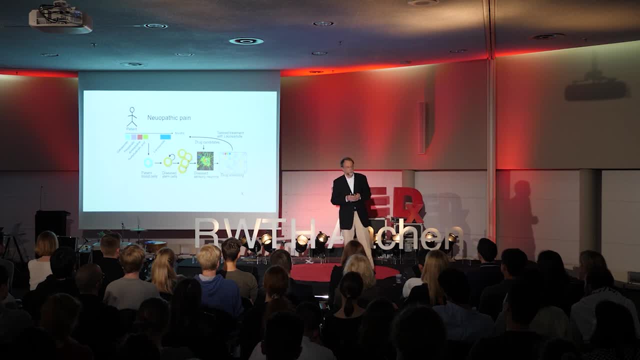 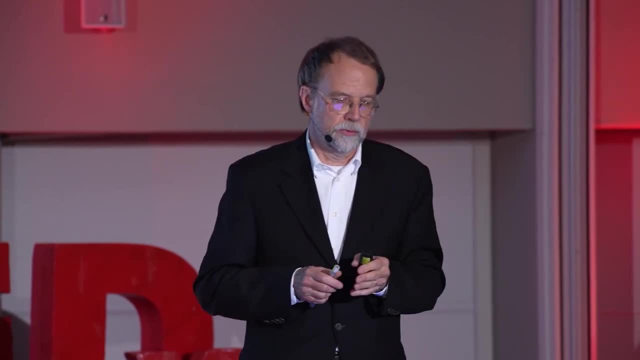 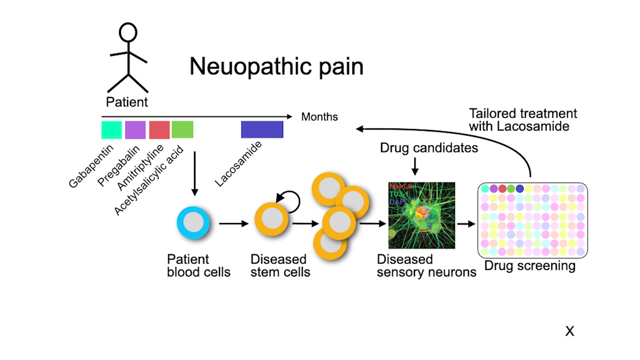 it was effective and it worked, So the patient is now without pain since many months. So this is a success story. But it's the same concept. So instead of using one drug after the other in consecutive treatments, we use a panel of drugs. 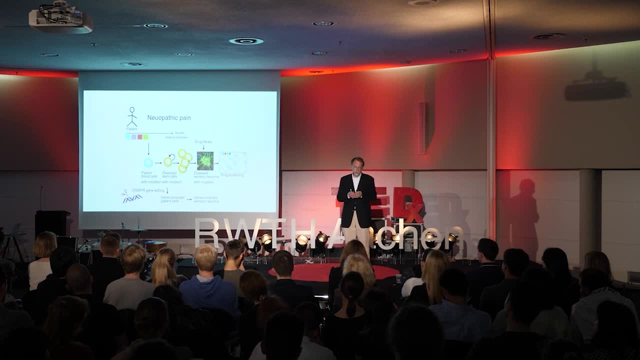 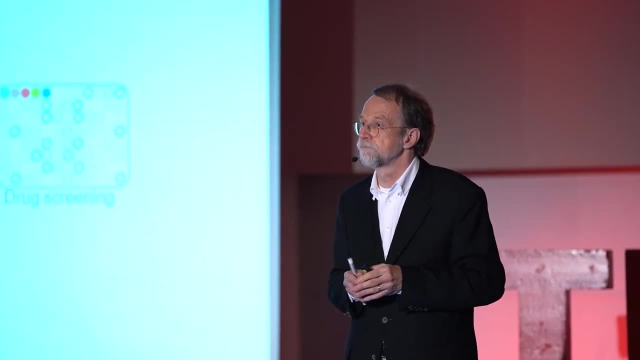 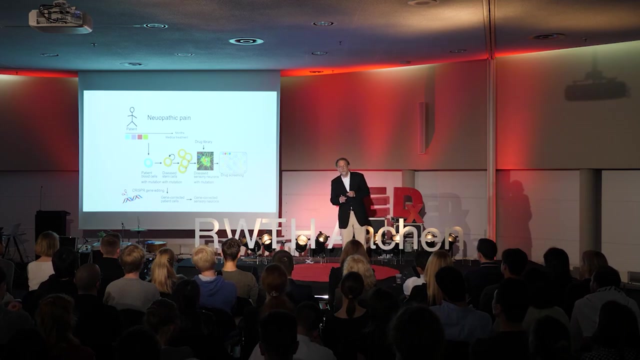 and screen for the panel of drugs to find a drug which would work in the diseased cells in the screen and then should also work in the diseased cells of the patient. But there is also a challenge because neuropathic pain comes with mutations. 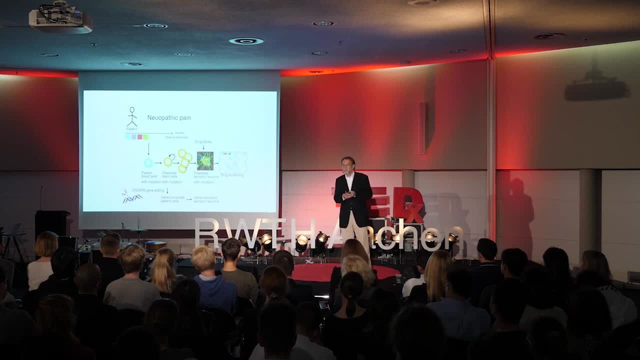 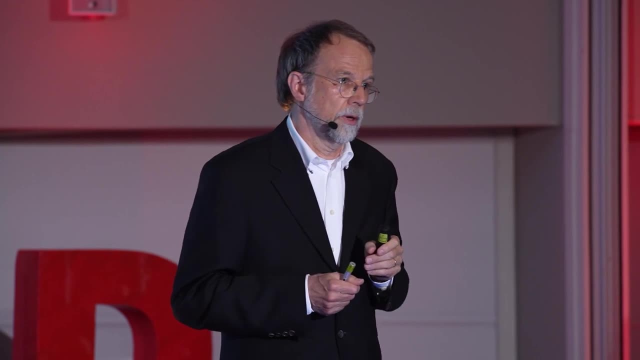 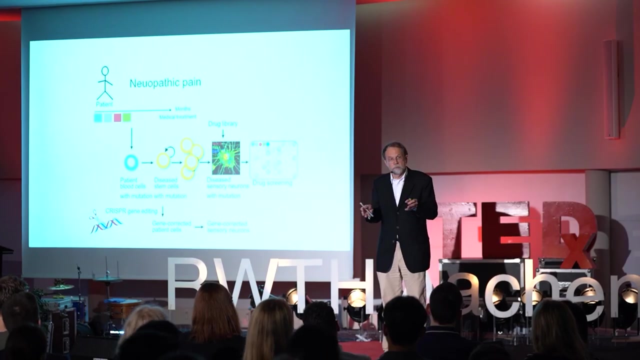 And these mutations are germ-like mutations. It means that they are in the family, So the mother of the father has this mutation and it's given to the kids, which means that all cells in this patient have this mutation. The mutation is only seen in the sensorineurons. 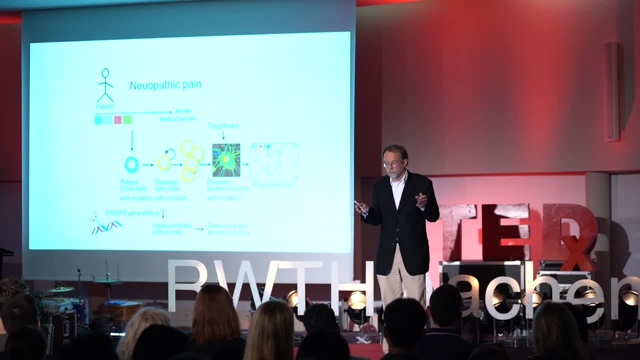 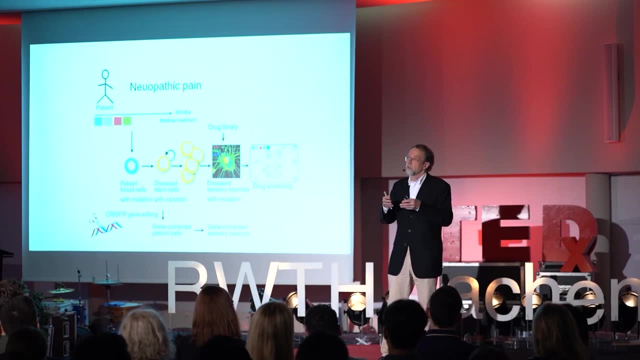 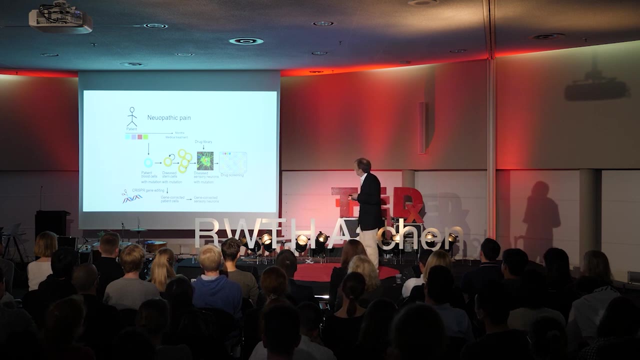 where the respective ion channel is expressed. But all cells have the mutation. So where do we get the healthy cells for our screening if all the cells have the mutation And there a CRISPR-1,, a gene editing, comes in. So this is a procedure. 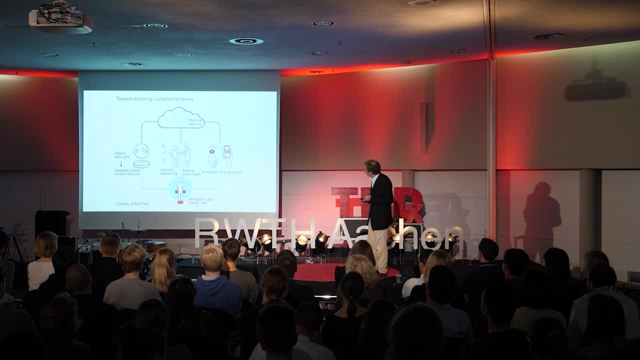 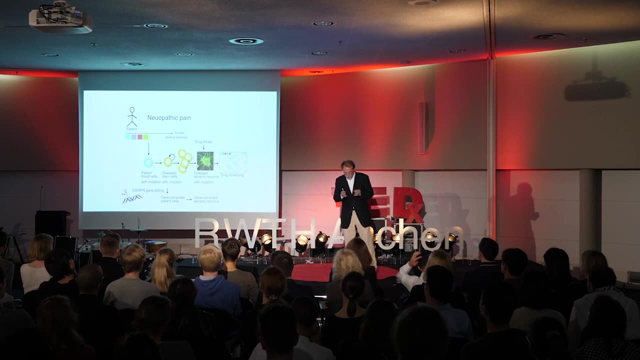 where we can repair, to go back where we repair the disease-causing mutation, Where we repair the disease-causing mutation and to generate now gene-corrected cells which are the equivalent of healthy cells. And CRISPR is a pretty simple procedure. 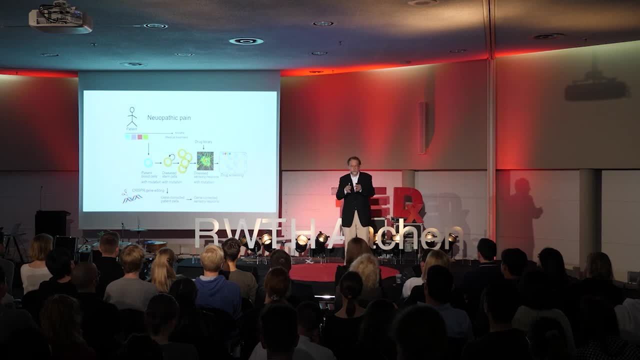 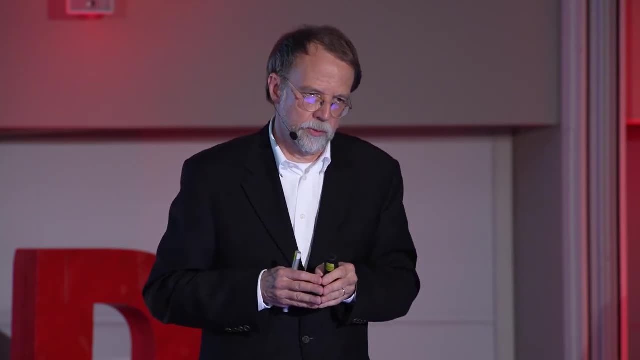 We have guide RNAs, a donor template, we have enzymes and we put this all together and then the DNA, the respective point mutation will be corrected. It's similar to a text editor you have on your computer where you use your cursor. 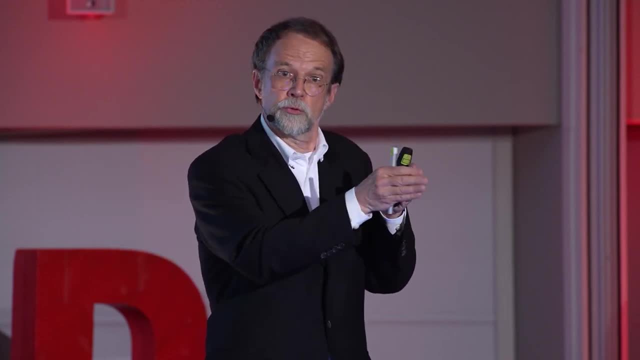 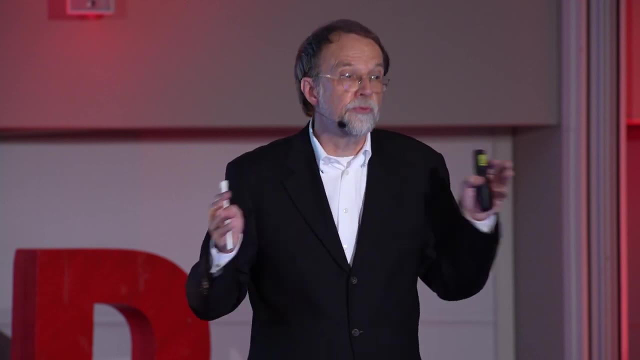 you move to the position where the spelling error is to correct the spelling error and it's done. And the CRISPR in stem cells is a particular versatile, a particular helpful combination, because it's sufficient to repair the mutation in one cell, one stem cell. 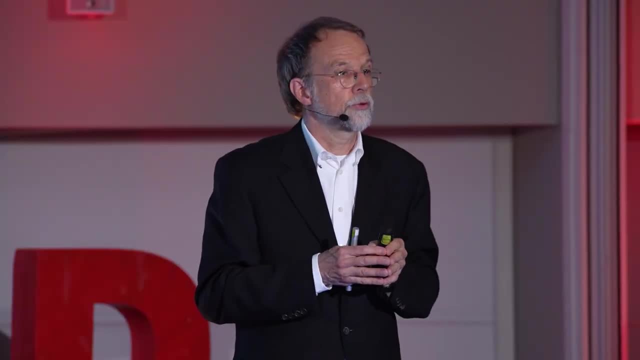 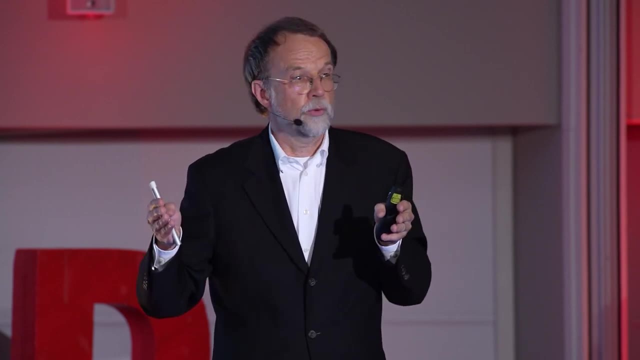 and then the stem cell can be amplified. It's similar if you were to correct the spelling error in the same text of 100 pages. So you can do this, of course, page by page, 100 times, or you just do it once in one page. 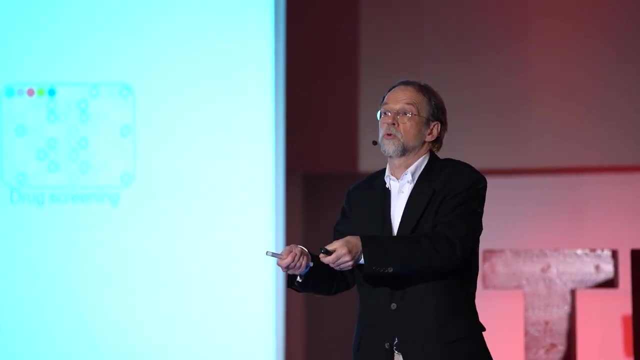 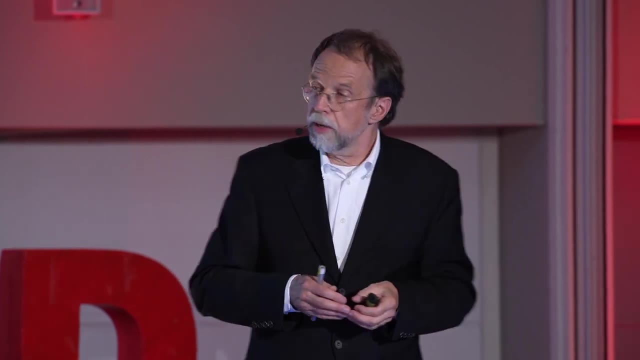 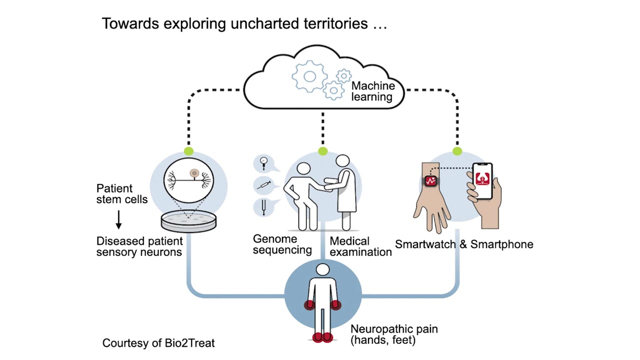 and then put this page in the photocopy machine to make multiple copies, or use the text editor to make multiple copies. Okay, So we would like to put this on higher level, And this is a study with a cohort of patients which have neuropathic pain. 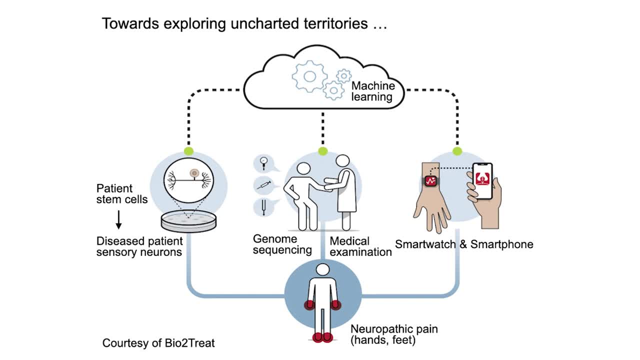 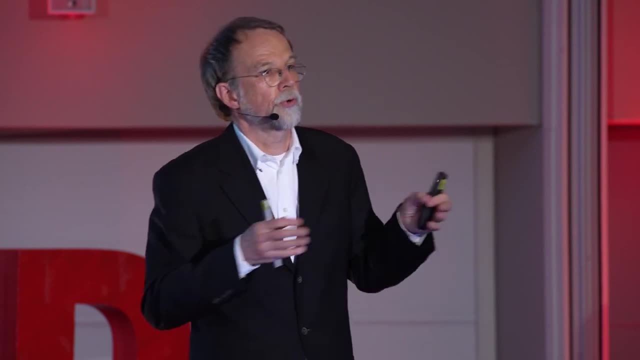 in the hands and feet, And we don't know so much about these patients, whether they have mutations, And so in this study, the patients receive a smartwatch and a smartphone, And the smartwatch would constantly record patient parameters and, say, heart frequency. 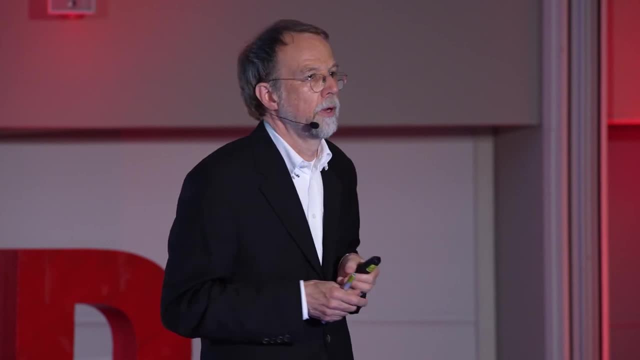 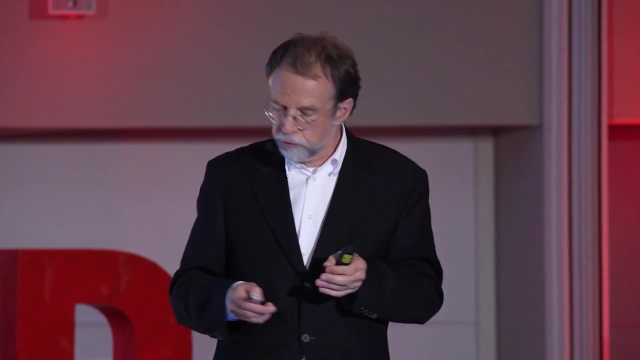 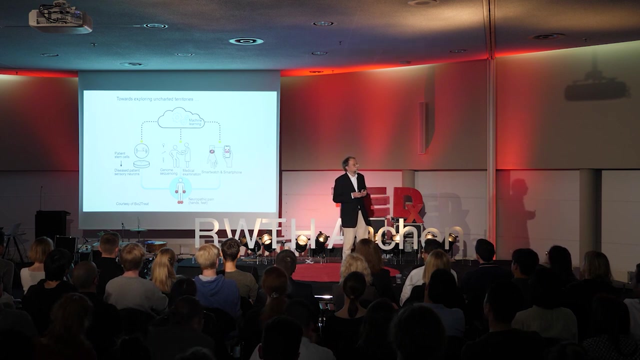 whether the patient is active, jogging or inactive. It would also record weather parameters- temperature, barometric pressure- And this all goes into the cloud. We would ask the patient also to report on his feelings in the smartphone. So how do you feel today? 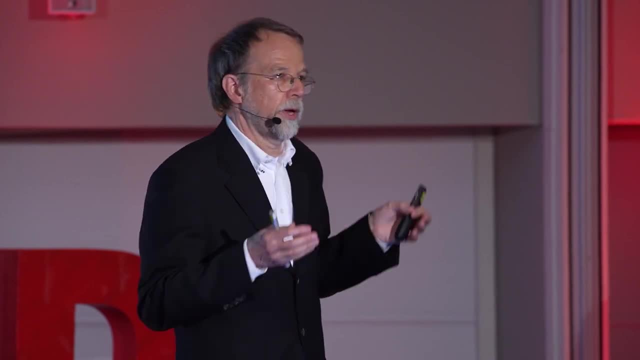 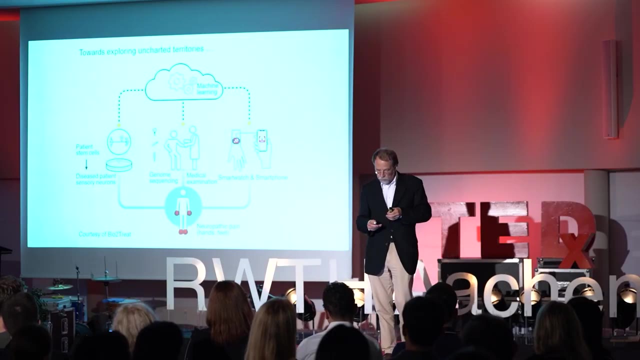 Did you sleep well? Did you have pain? Was it long-lasting pain? Was it sporadic pain? How would you judge your pain on a scale from one to five, And this information also goes into the cloud. Okay, The patient would also. 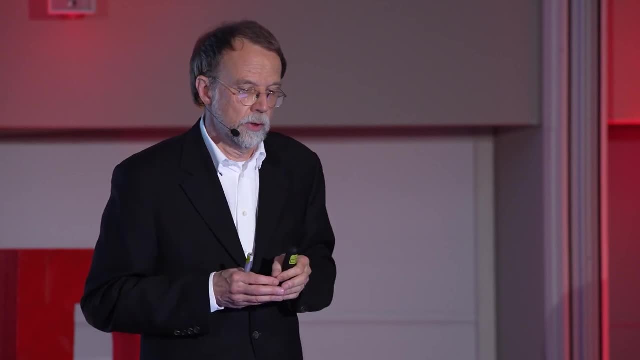 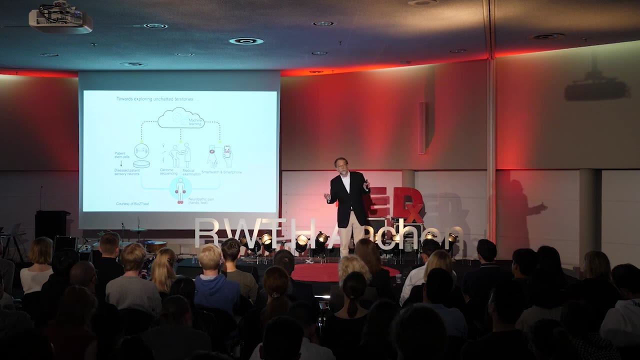 see the medical doctor in regular time intervals and will be subjected to medical examination. This information also goes into the cloud. Also, a blood sample will be taken. Normally this is very well accepted by patients when the blood sample is taken And this blood sample 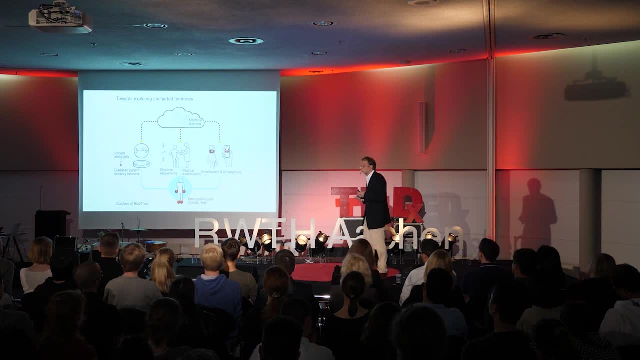 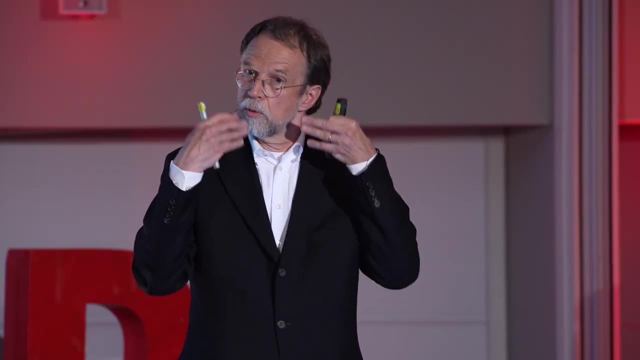 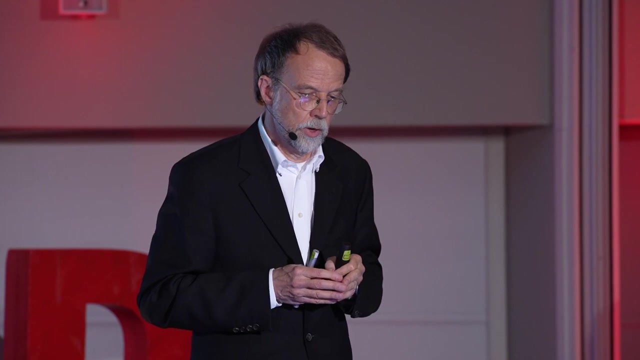 is used to prepare DNA for genome sequencing. We suspect that these patients have mutations, but we don't know where And we need to find them, So the objective is to determine the complete nucleotide sequence of the patient and to see whether there are mutations. 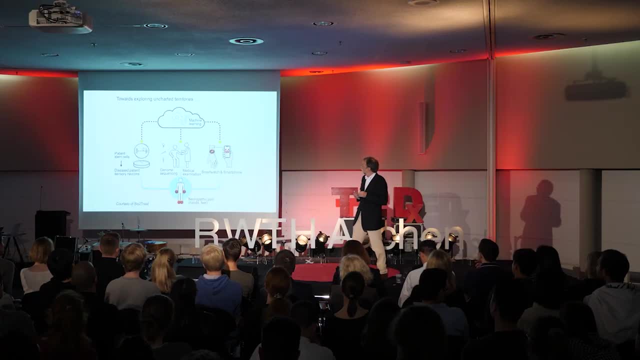 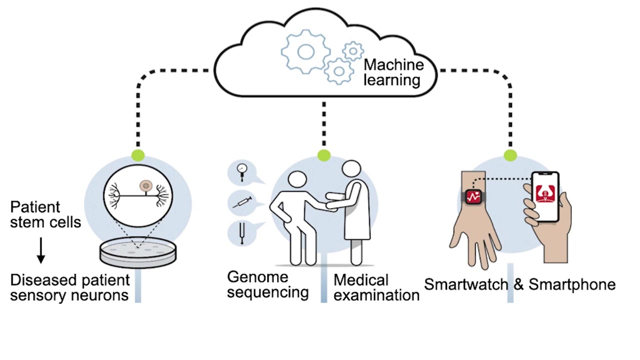 And this blood sample is also used to prepare patient stem cells and disease And the biological readout is also put into the cloud And we then use machine learning to relate the data from the patient, from the medical examination, and the biological data. 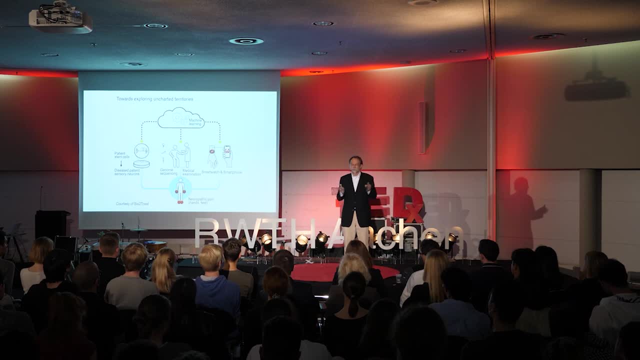 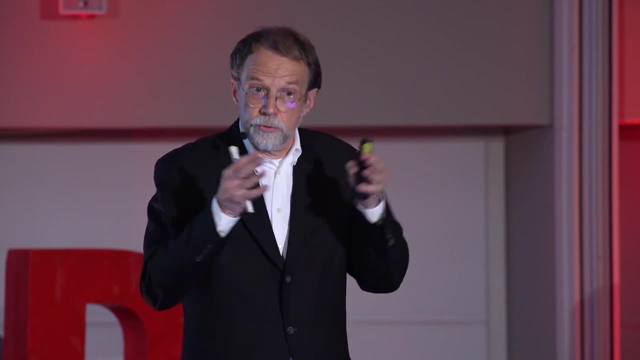 and see whether there are overlaps, there's coherence, whether the mutation is now being possible to be identified. So this is an ongoing study. We're very excited about the results. We don't know the result yet, but we are very confident that this is a very important 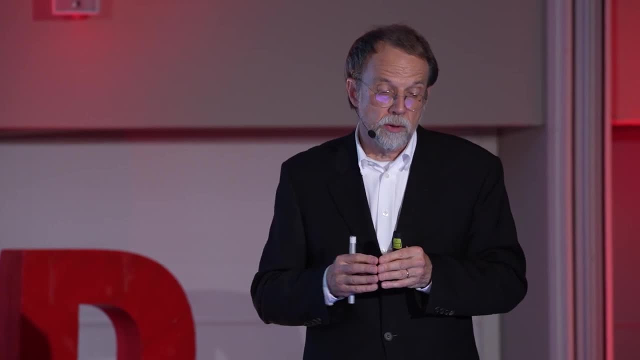 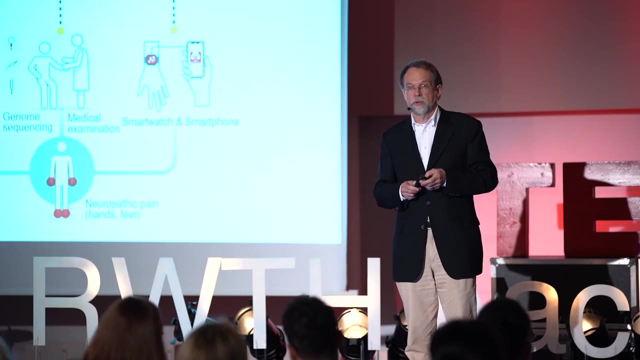 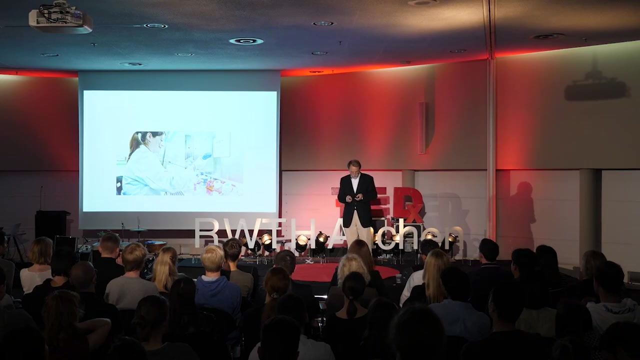 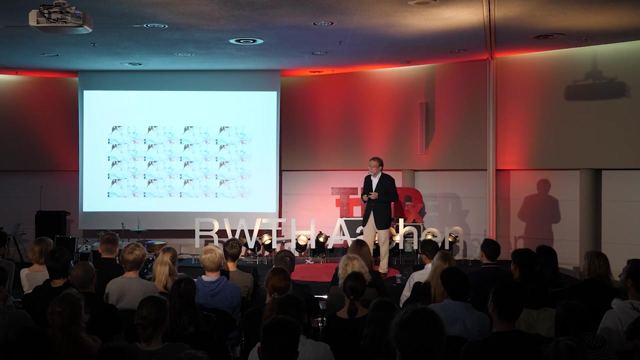 and future-directed study. What we also need to address is upscaling. So, working with patients, it means not working with only one patient, but with several patients, And this is to address upscaling. This cannot be simply done by increasing the number of people in the laboratory. 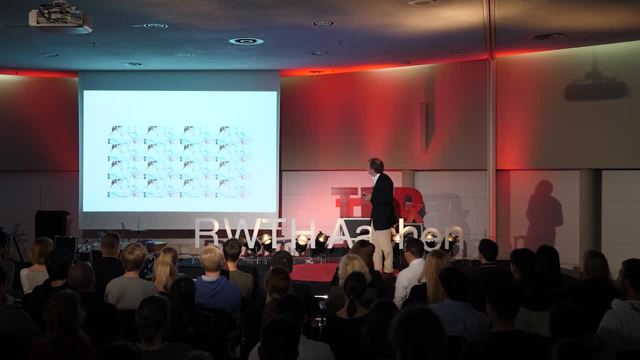 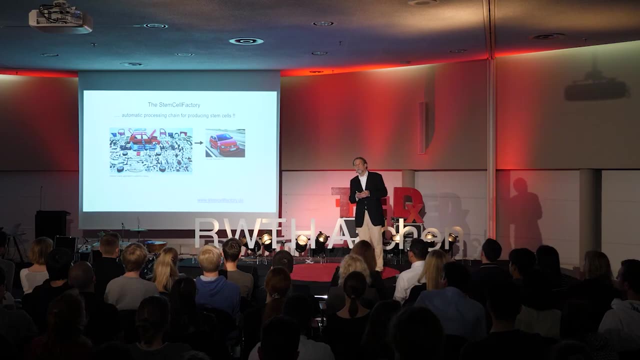 And we do this by moving into robotics and have a system which we refer to as stem cell factory, which is a system which is an automatic processing chain for producing stem cells. It's similar to a car factory, where all the items you need for a car 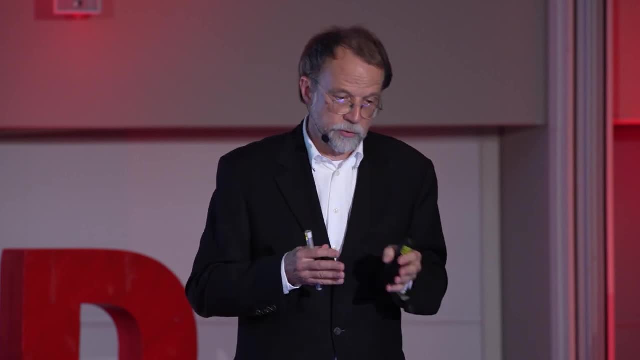 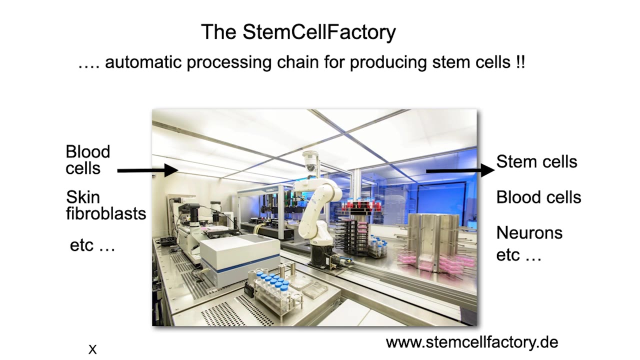 are put together to generate a car, But the items being put in these stem cell factory are, of course, different. So blood cells, fibroblasts, biologicals, and the output is also different. We have stem cells and blood-derived. 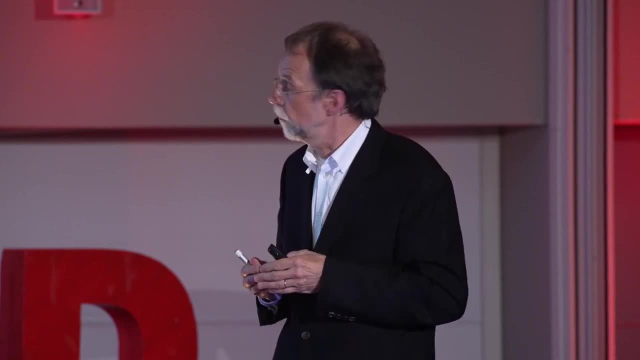 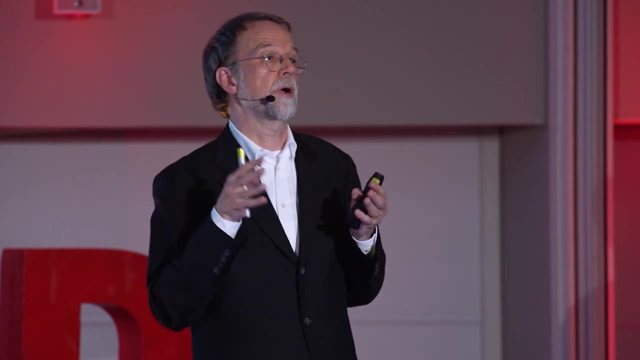 stem cell-derived products like blood and neurons and so on. So we are very enthusiastic about this project and it's really funny to see the robot rushing around grabbing a plate and putting it in the microscope or getting it in the incubator or the liquid tank.